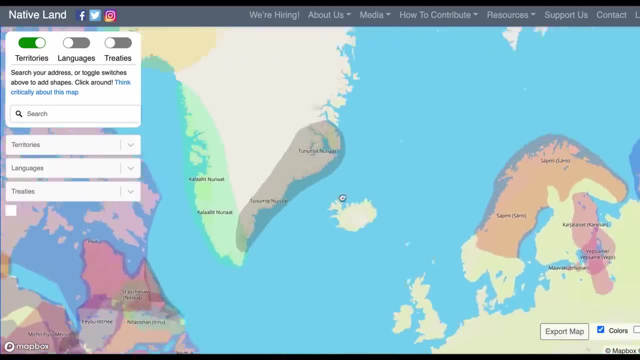 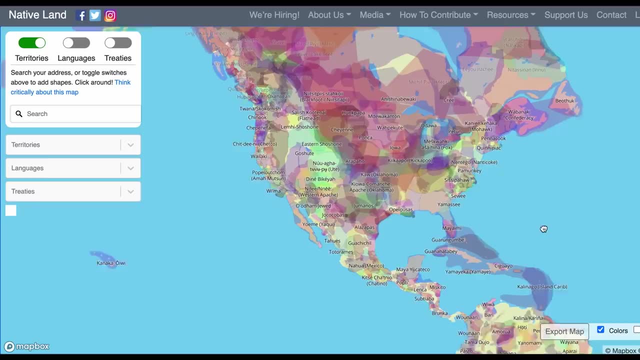 Greenland, Scandinavia and parts of Russia and much of South America which is still being put together. If you've seen any videos in the US Explained, a series where I make a video on each state, territory and federal district in the country, you might recognize this interactive map. 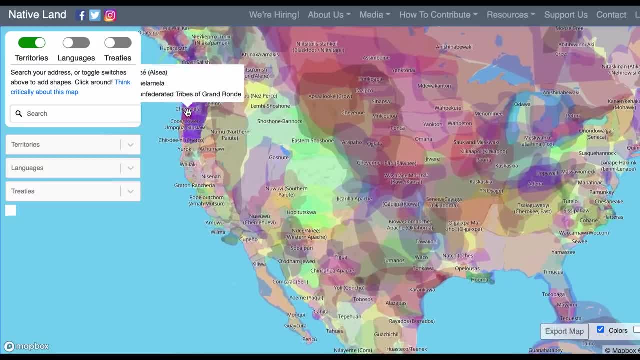 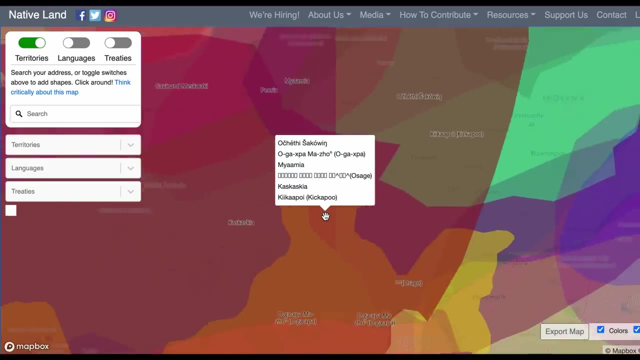 which I've used to determine the indigenous peoples whose homeland sits in each state. It includes a button to turn on labels which overlap the map with modern political boundaries, cities and towns. This can be a helpful way to find where you live and learn more about the native people whose ancestral land you. 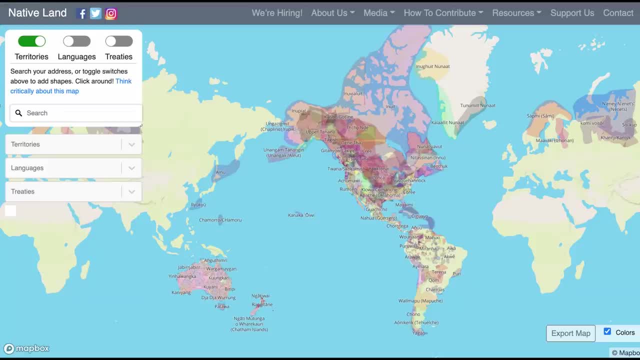 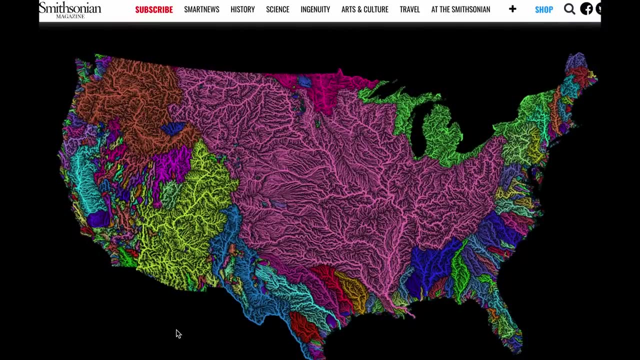 reside in Nativelandca is a very interesting map that I definitely recommend you check out. Next up is a series of maps created by Hungarian mapmaker Grasshopper Geography. It splits the world up into different watersheds, basins in which all precipitation eventually drains. 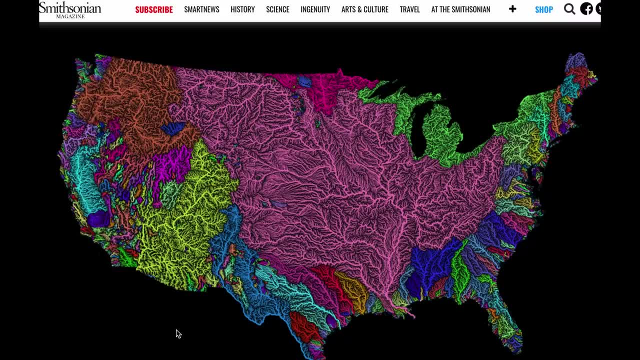 to the same place. These are just fascinating to look at. You can see that coastal areas are split into tons of tiny watersheds, usually smaller creeks, that start in areas not far from the sea, whereas inland single watersheds, like that of the Mississippi, can take up vast swaths of land. 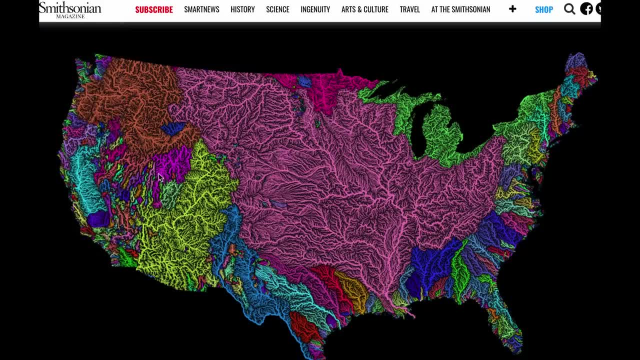 In drier, more mountainous areas, some valleys may be completely cut off from the ocean and not receive enough rainfall to fill up into lakes that then get large enough to overflow, creating what are known as endorheic basins, areas where rivers flow into lakes that 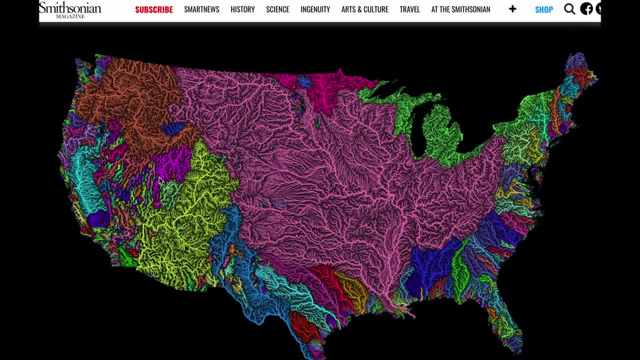 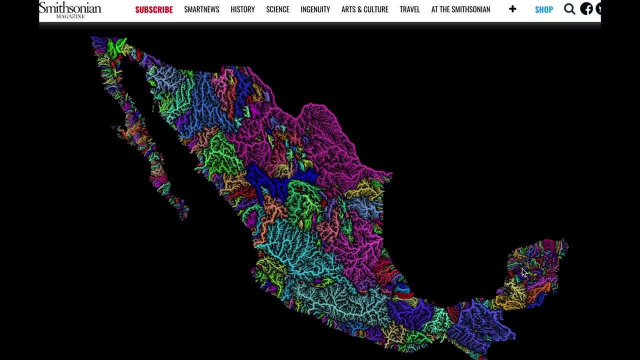 then go nowhere with water leaving through evaporation in the hot desert sun. You can see plenty of these in hot desert areas like Nevada and much of the US's Mountain West. In the Yucatan Peninsula of Mexico, a large inland section is home to a bunch of self-contained 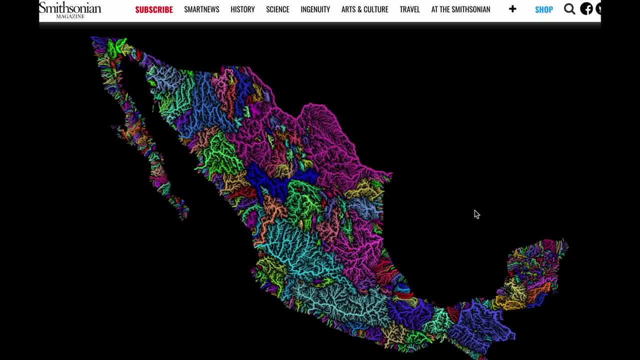 watersheds as well, Despite it being flat and having plenty of rain, unlike other mountainous desert areas where that is not the case. I'm guessing that this is due to the presence of cenotes, which are essentially sinkholes that have filled up with water and are super common in the region. 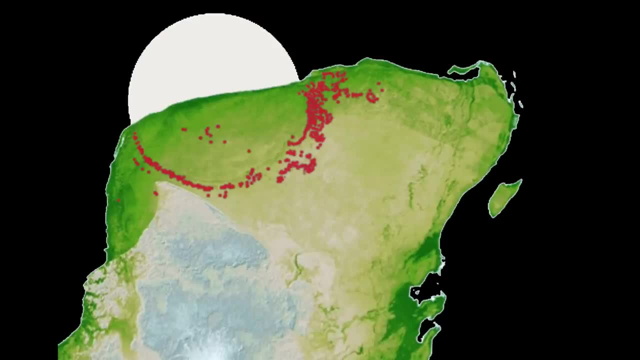 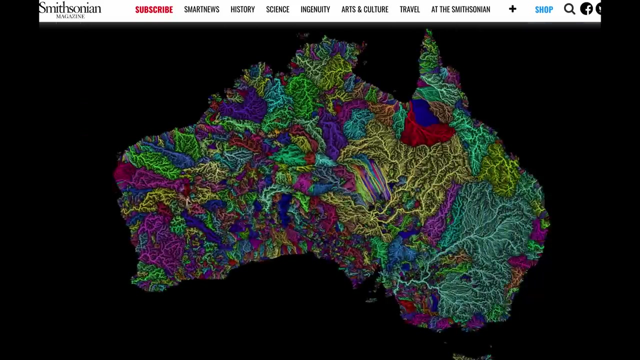 Many are located in an enormous ring marking the edge of the Chicxulub Crater, the location where the meteor that brought an end to the dinosaurs struck the earth. There are plenty of incredible watershed maps to see here. The outback of Australia is dotted with too many. 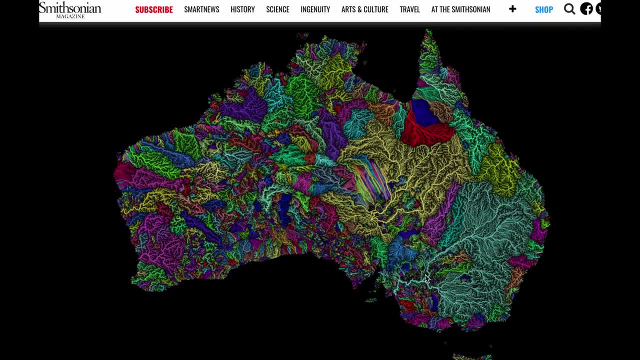 self-contained evaporation basins that count, including some that sit right next to rivers. I'm also very curious about what's going on right here, so if anyone from Australia knows why the watersheds in this section are all in straight lines, leave a comment below to let me know. 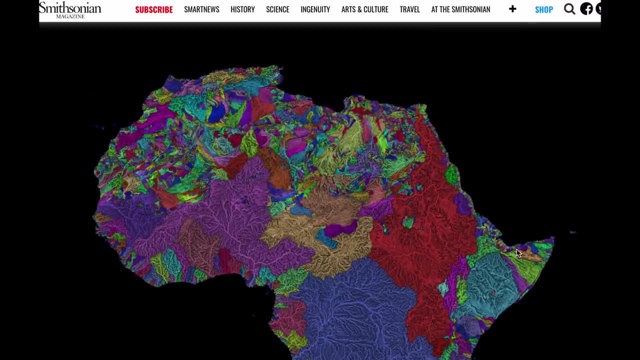 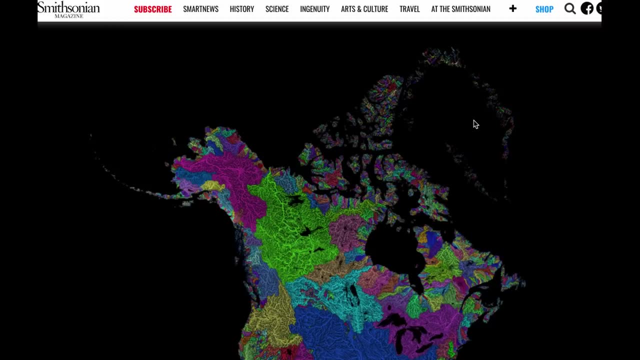 The Sahara, too, looks really impressive on this map, as does Greenland, which, due to the presence of its vast ice sheet, only the outline of is visible. There are plenty of places to see these watershed maps. I found them on the Smithsonian Magazine and I definitely encourage you to check them out. 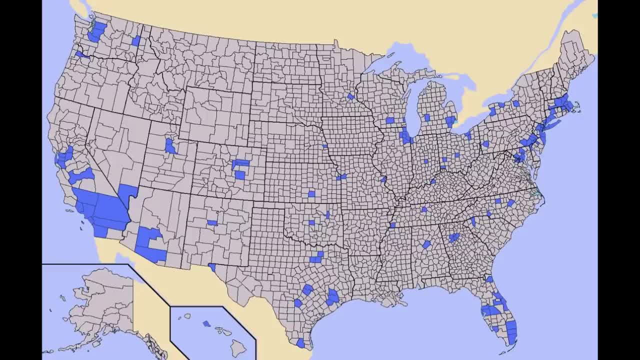 The next map is made by Business Insider and it is pretty mind-blowing. It shows the US broken down by county, but the blue counties that have been selected are home to half of the country's population and the grey counties home to another half. This is just a fascinating way to visualize. 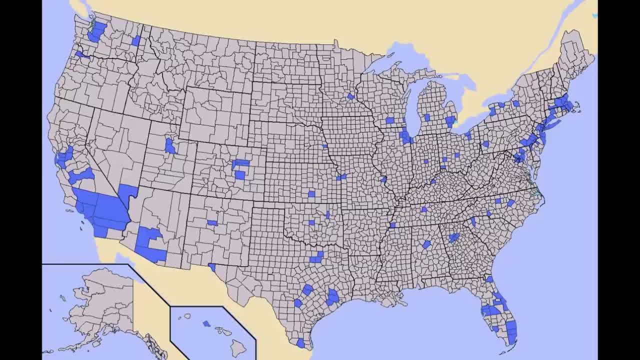 the differences in population density between urban and rural areas. Even though two counties may take up the same amount of land, some may be home to only a couple hundred residents, while others may be home to millions. If you live in the US, take a look at this map. I imagine many of you 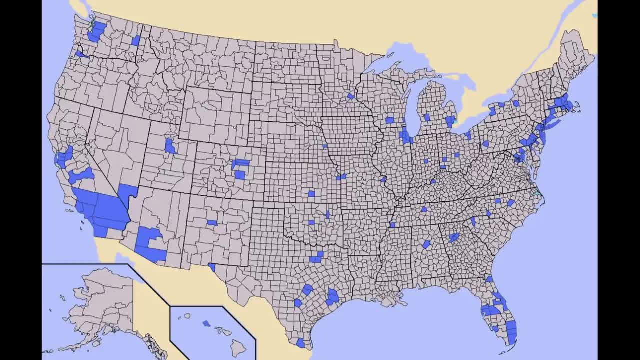 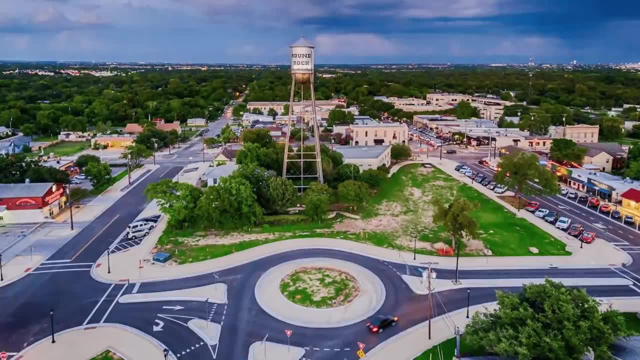 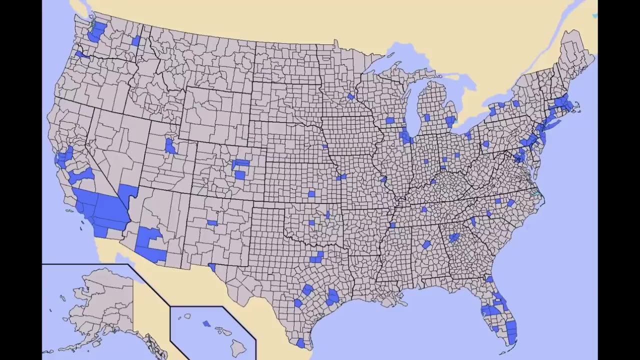 live in one of the 146 highlighted counties, which range from Los Angeles County in California, home to a stunning 10 million residents, to Williamson County, Texas, and Bourbon County, to the north of Austin, home to almost 600,000.. Leave a comment below if you. 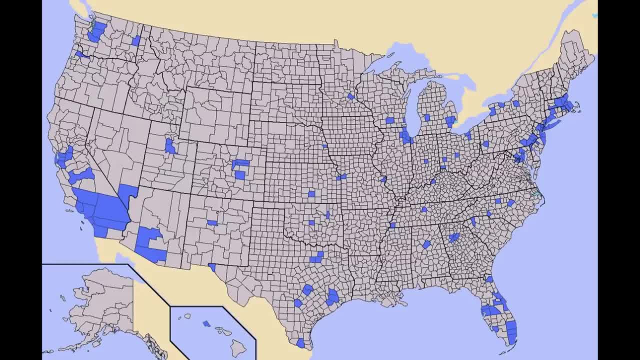 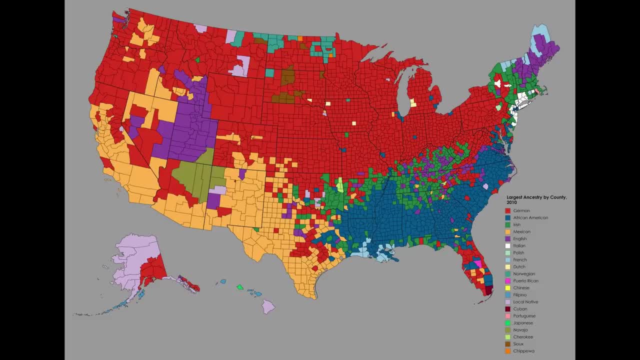 live in one of the highlighted counties and be sure to check out this map. This map, which I found on Vivid Maps, depicts the counties of the US, broken down by the most common country or ethnic group the ancestors of its residents were part of. This is interesting because it shows clear patterns. 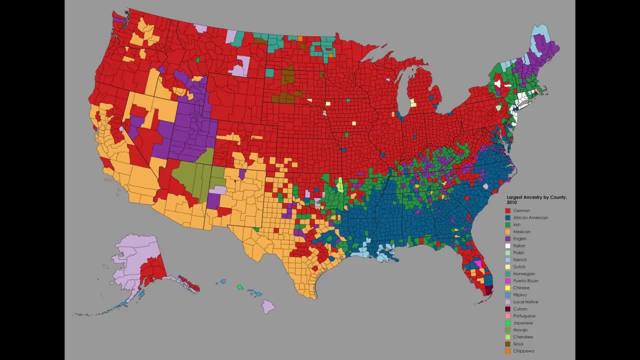 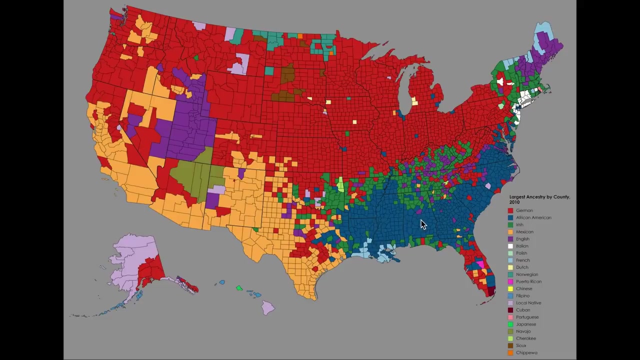 in how immigrants settled in the United States, often choosing to live alongside people from the same country who spoke the same language. In addition, the population patterns of some ethnic groups in the US were a result of force: Black Americans, many of whose ancestors were forcibly enslaved, and 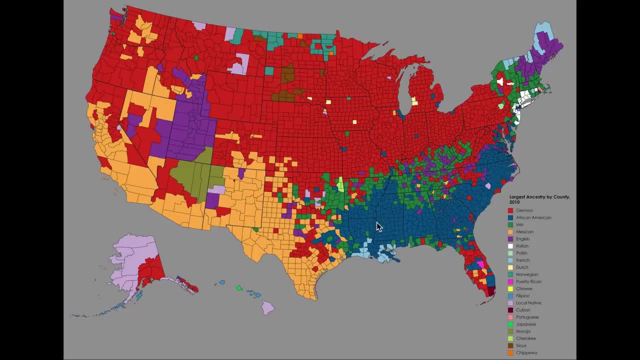 brought to the country in chains are today the predominant ancestry group across many counties of the southeastern US where the evil practice of slavery was most prevalent, as well as in many northern cities where millions fled during the Great Migration moving north to escape the 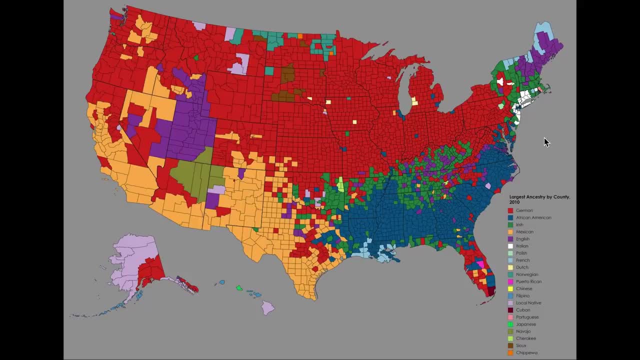 persecution of the Jim Crow South and seek better job opportunities that opened up during the World Wars. In the Western US, many counties are majority Native American. For the most part, these are locations of reservations, such as the Navajo Nation in the southwest, But you'll notice that there are only one or two such 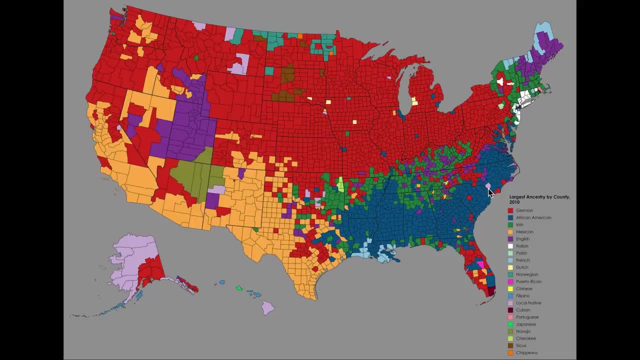 majority indigenous counties in the eastern US. Most native people that survived the spread of diseases brought from Europe, like smallpox, as well as the genocidal practices of colonial expansion, were often forced away. The majority of the population in the western US are Native. 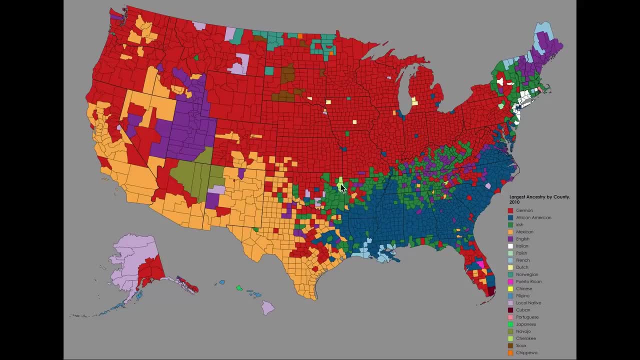 Americans In the southwest, such as the Cherokee, who make up the largest ancestral group in several Oklahoma counties, but whose homeland is located in the southeastern part of the country, in states like Georgia. In terms of immigrant groups, you can see that many residents of the 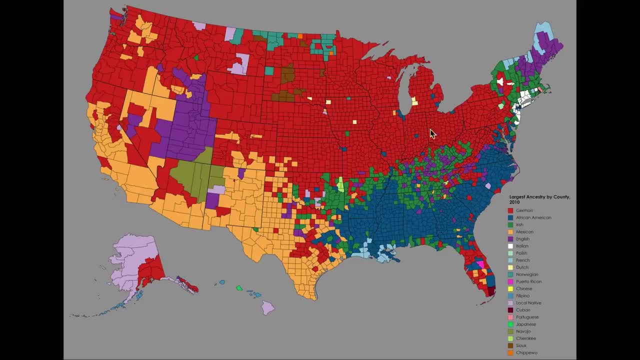 northern United States, especially in the Midwest, are descendants of German immigrants. In fact, German Americans make up the largest ancestry group overall in the country: 16.4% In the southwest and mountain west. residents of many counties like Massachusetts and New York are descendants of immigrants from Mexico And descendants of 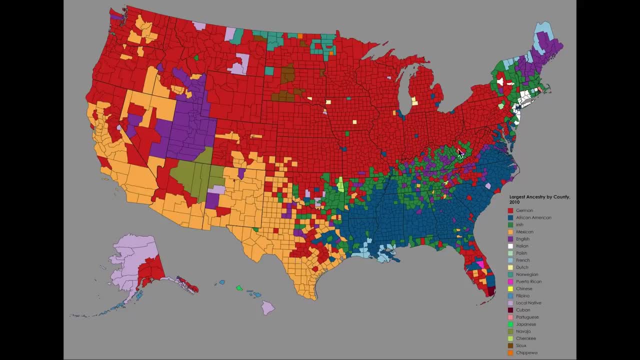 Irish immigrants inhabit parts of the south, alongside northeastern areas like Massachusetts and upstate New York. There's also one county way out in Montana that I'd be interested in knowing the story behind For a country dominated by the English language. you'll probably be. 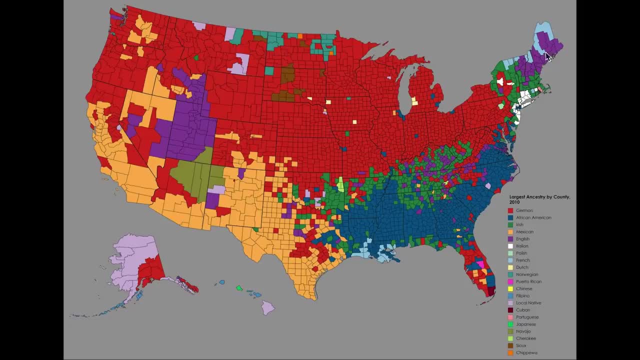 surprised to see that in few parts of the country are most people descended from English immigrants, mostly the upper New England states and parts of Utah and Idaho. due to the fact that most Mormons members of the LDS church are of English descent, French ancestry is dominant in. 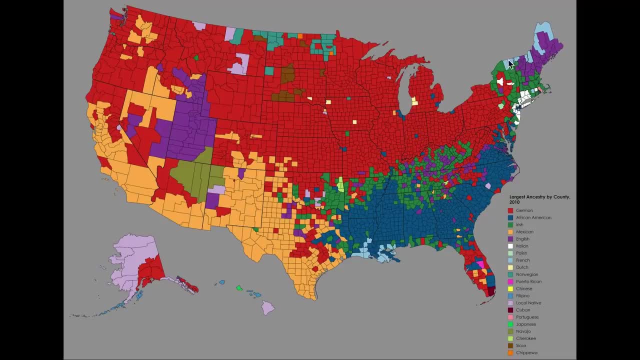 the rural parts of upper New England that border Quebec, as well as in parts of Louisiana, which has a long French history. Many descendants of Italian immigrants live in the New York metro area and many people in the rural upper Midwest trace their ancestry to immigrants from Norway In San. 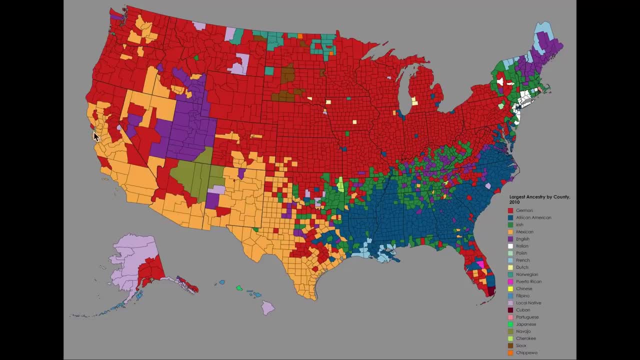 Francisco, which acted as the historic gateway to immigration from East Asia. more residents have been born in other countries And many people in other counties along the Pacific coast trace their ancestry to immigrants from other Asian nations such as Japan and Hawaii and the. 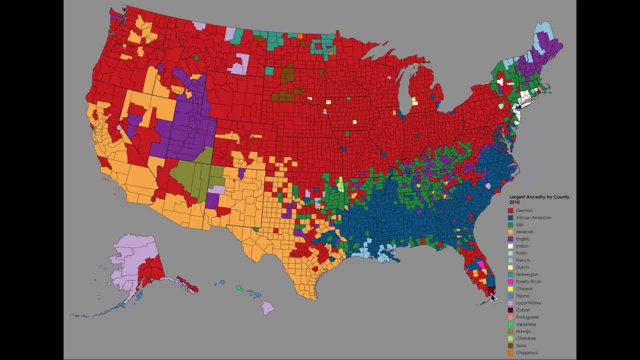 Philippines and Hawaii and Alaska. Residents of Miami-Dade County in Florida are predominantly of Cuban descent, and residents of another county in Florida are primarily Puerto Rican. Luzerne County in Pennsylvania is the only mostly Polish-American county in the country, and Bristol County in Massachusetts is the only mainly. 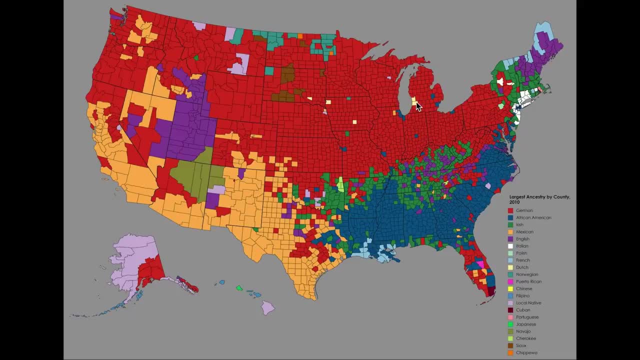 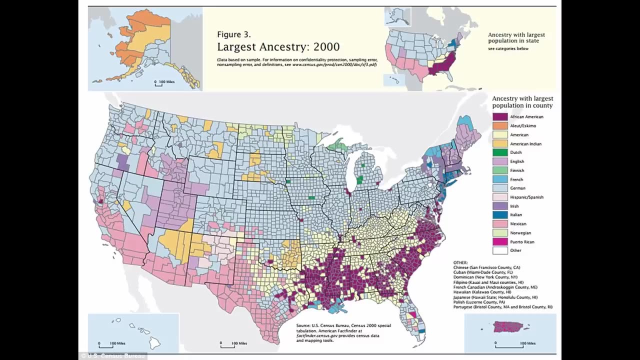 Portuguese American one. You can also find some counties sprinkled throughout the Midwest where most people's ancestors came from the Netherlands, and I've seen other maps that show the upper peninsula of Michigan as having a large Finnish American population. This map is a fascinating 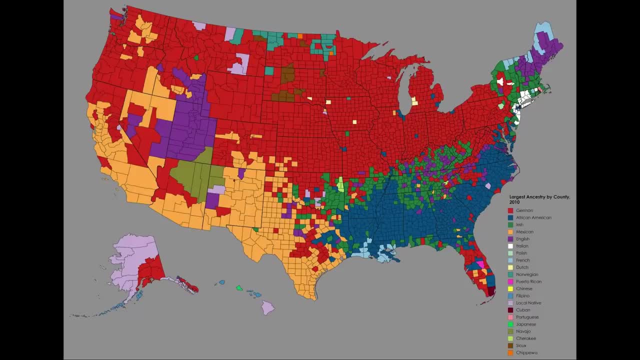 way to visualize how immigrants to the US often settled, and continue to settle, near one another and the impact these different communities have had on shaping the country we know today. Also just for fun, this map made by Maptitude does the exact same thing, but depicts it using 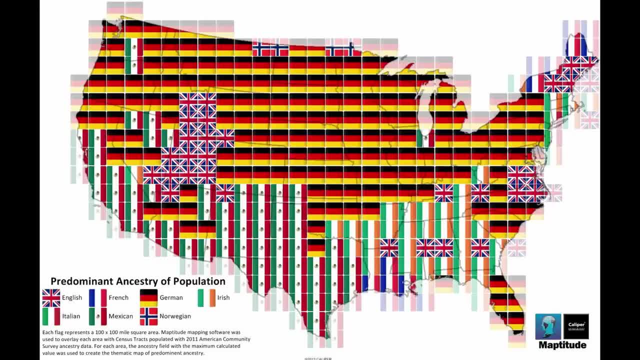 flags, so it is less detailed but creates an interesting visual element. It was shared on my Discord server, so if you're interested in seeing more fascinating maps like the ones I'm showing in this video, then please feel free to join. I'll put the link in the description. 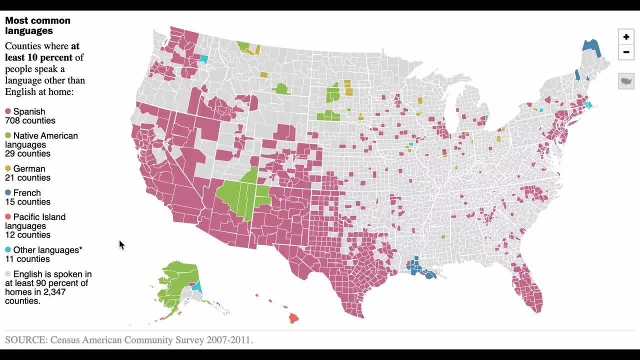 The next map builds off of the last one. It's an interactive map made by the Washington Post that shows every county in the country in which at least 10% of households speak a language other than English. at home, Spanish is most common, but other areas have. 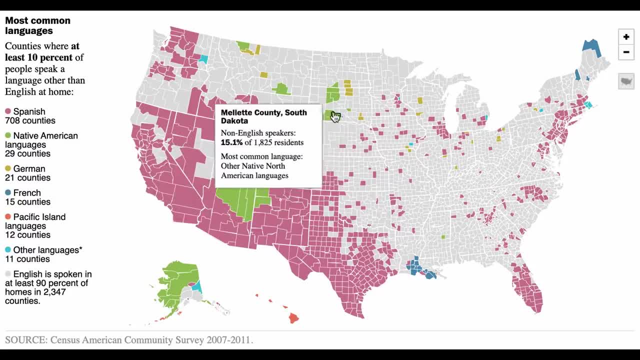 large populations that speak indigenous languages along with French, Chinese, German and other languages at home. It does a great job depicting the various linguistic communities in the US and serves as a strong reminder that, despite the prevalence of English in public life, 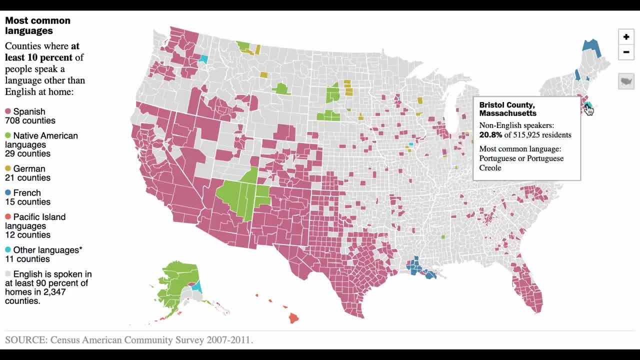 the United States is very much a multilingual country. The final map I'll discuss in this video is called an extremely detailed map of the 21st century. It's a map of the United States, and it's a map of the United States. 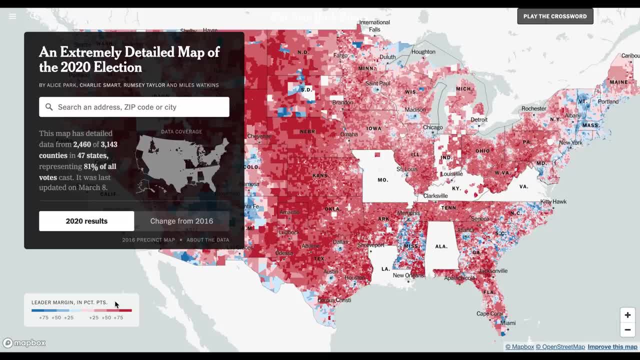 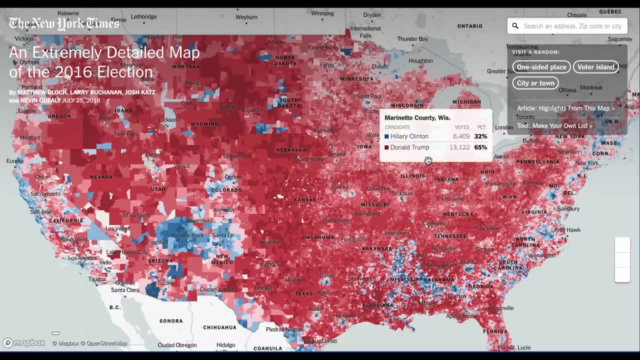 It's a map of the 2020 election made by the New York Times. It's a follow-up to a map I discussed in my Fascinating Maps video, which did the same for the 2016 election, Just like the map in that. 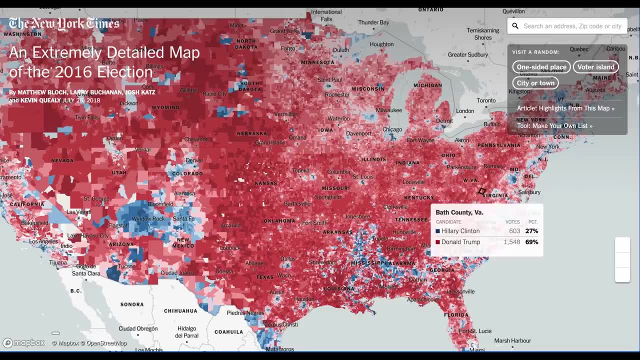 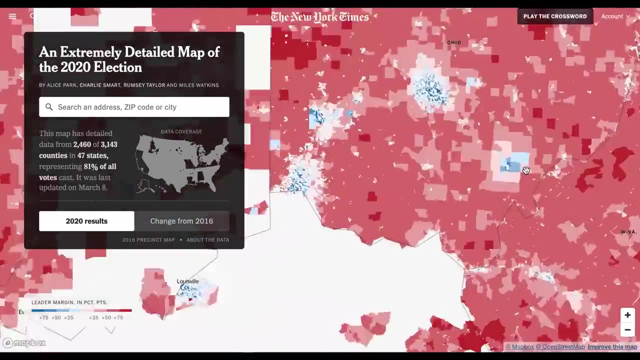 video. this map shows how the country voted down to the last precinct. This makes it far more detailed than other electoral maps, which typically show voting patterns by state or even county. Just as with last time, maps like this can be pretty misleading. There's a lot of red. 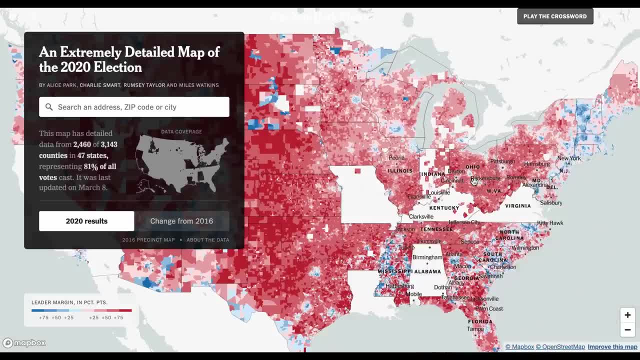 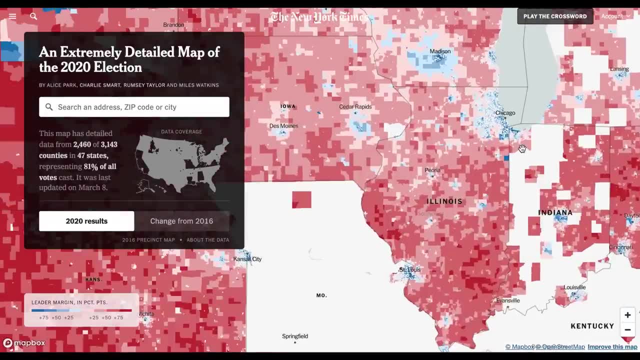 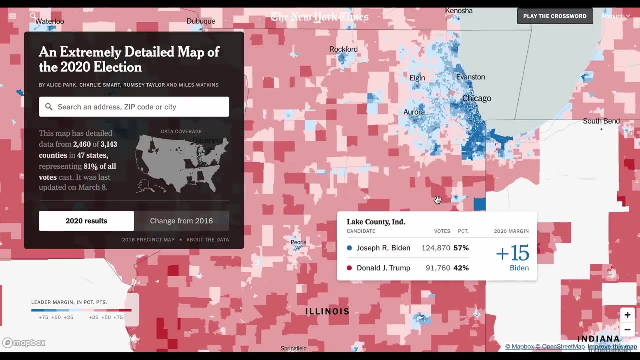 far more than there is blue on the map, but in reality there are pretty similar numbers of Republicans and Democrats on the country, and elections rarely ever are a landslide, especially in the popular vote. On top of that, 2020,, of course, saw Biden, the Democratic Party's nominee, win the presidency. 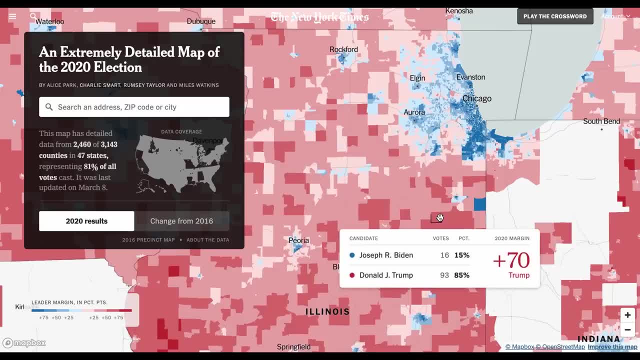 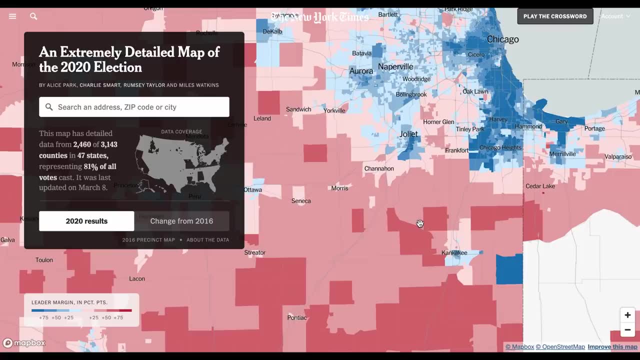 The reason that so much land on the map is colored red is due to the urban-rural divide that plays a major role in US politics, with voters in cities typically supporting Democrats and voters in rural areas usually supporting Democrats. So the map is a map of the 2020 election and it's a map of the 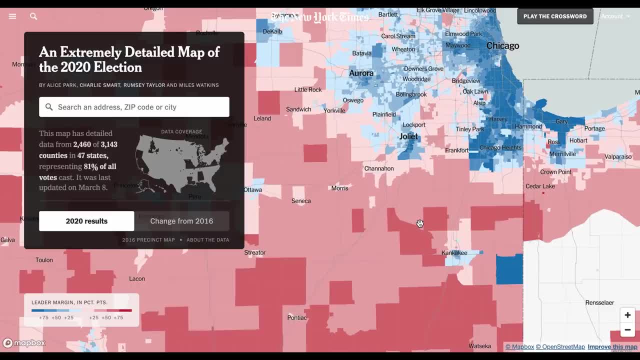 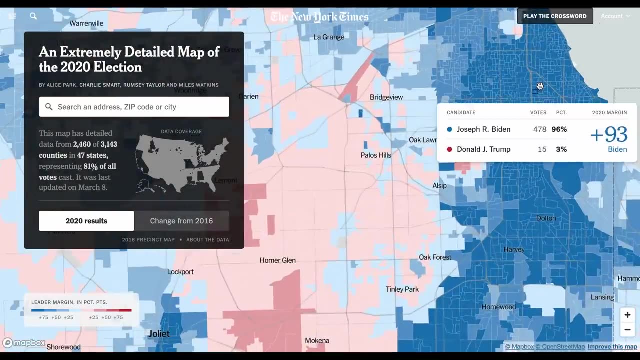 potential Precincts in rural areas are often home to a couple hundred voters and tend to vote red. Move into a city, however, and the precincts become not only smaller but bluer, and are usually home to a similar amount, if not more, of voters. Long story short. while there are about 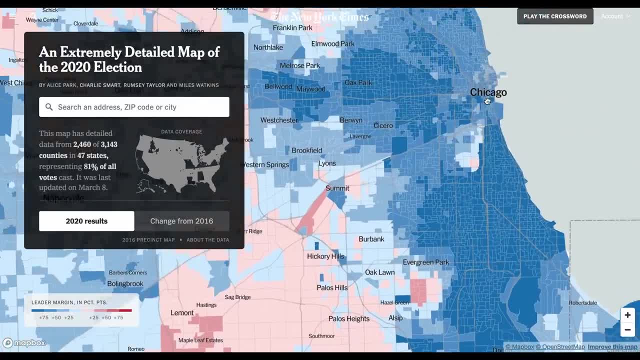 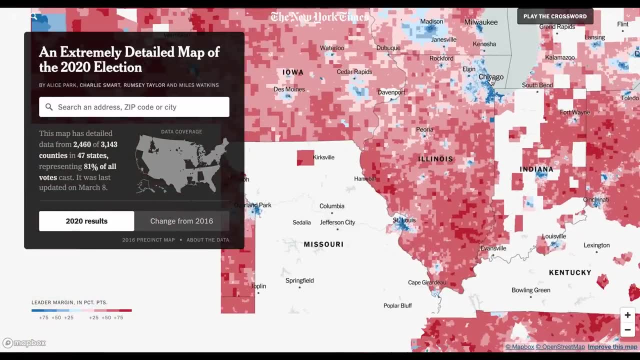 even numbers of Democrats and Republicans in the US. Democrats tend to live in more densely populated areas, whereas Republicans tend to live in more sparsely populated ones. There are some maps that take that into account, such as this one, which warps the physical size of states so they 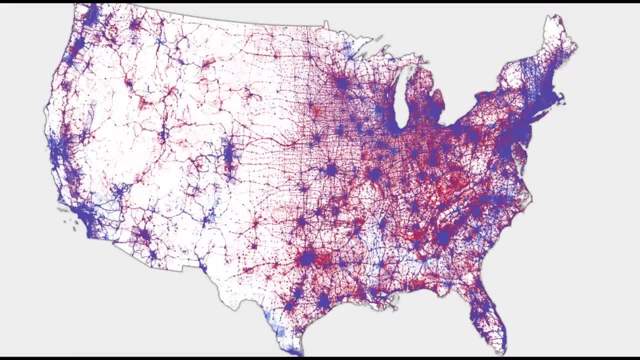 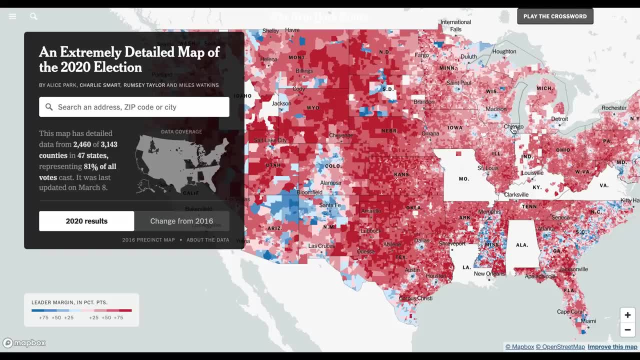 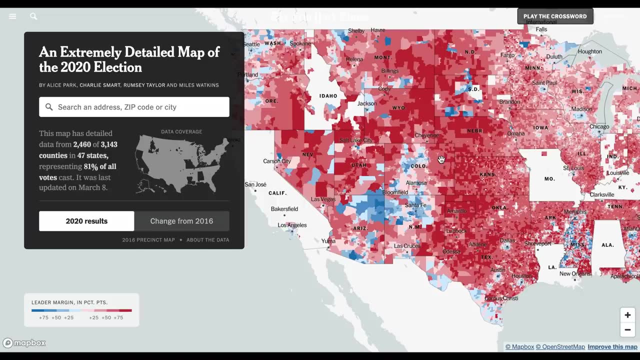 are proportional to their population, or this one which shows one dot per vote. in the last maps video, i focused on areas that did not follow the urban- rural divide, and in this one i'll focus instead on the potential long-term political trends that this map shows. first off, a couple. 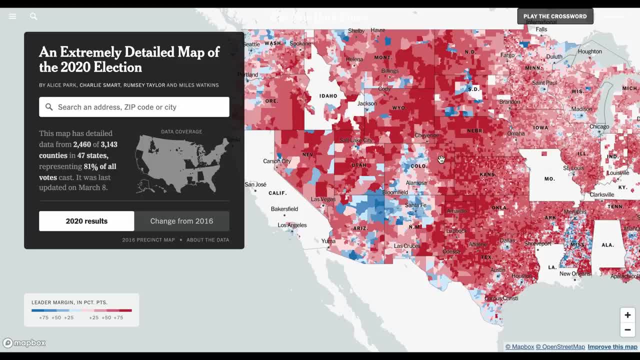 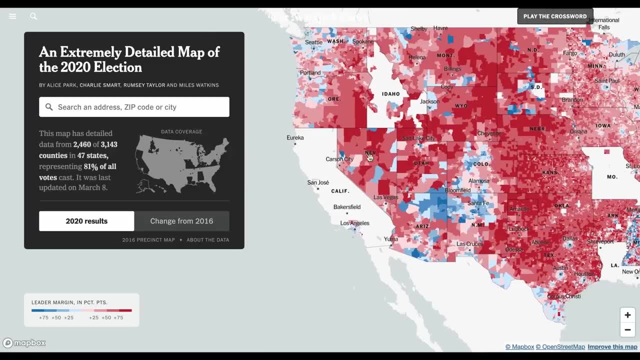 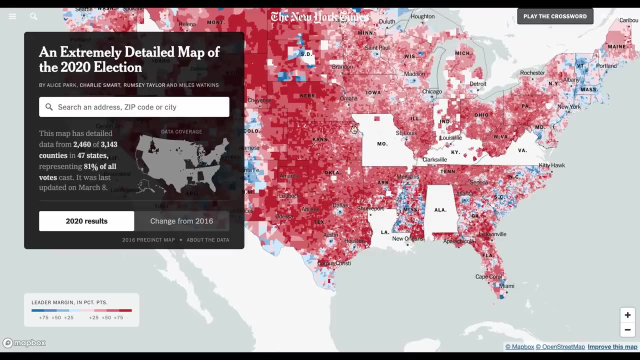 things about this map one. as of now it's only 81 complete. i don't blame them. props to whoever's working on this, because making a map this detailed looks incredibly difficult. but as time goes on, they've been able to fill in more and more, and we can still get a lot from what there is already. 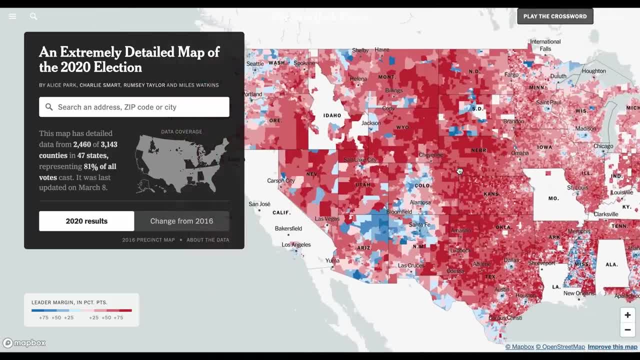 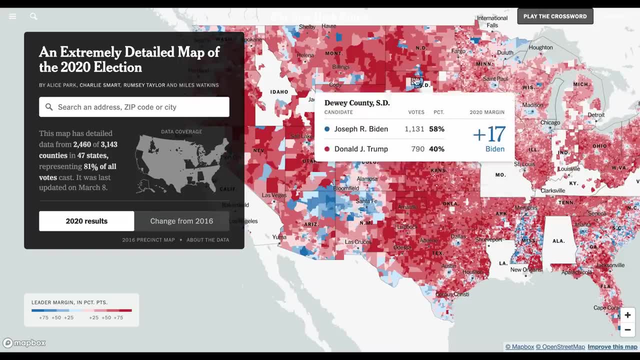 it's also generally more user friendly than the last one. when hovering over counties or precincts, it calculates and displays for you the margins. the respective winner won each buy, which is just a nice touch. in addition, it contains a button that allows you to toggle between it and 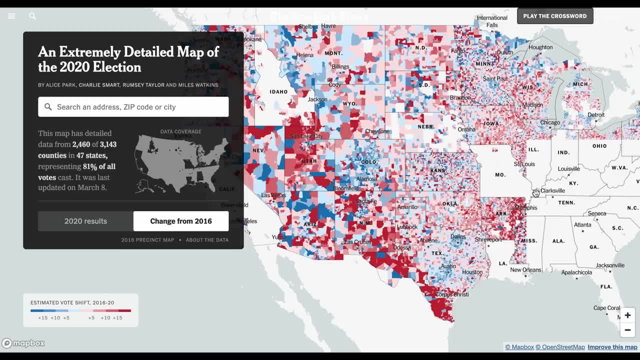 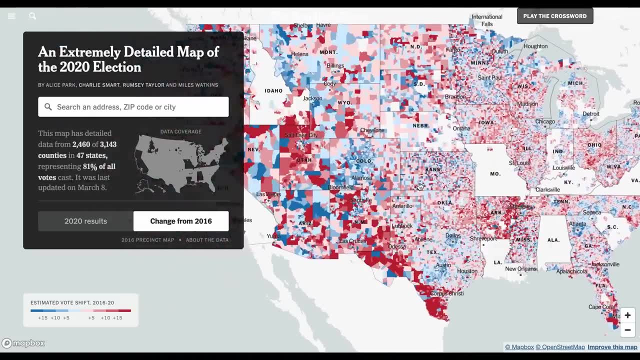 another map, one which has calculated the differences between the map and the map, one which is just a nice touch- in addition, it contains a button that allows you to toggle between it- and another map, one which has calculated the differences between the map and the map and shows whether that specific precinct or county has trended either more republican or more. 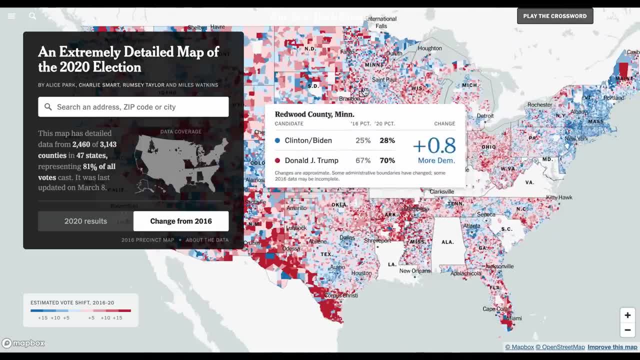 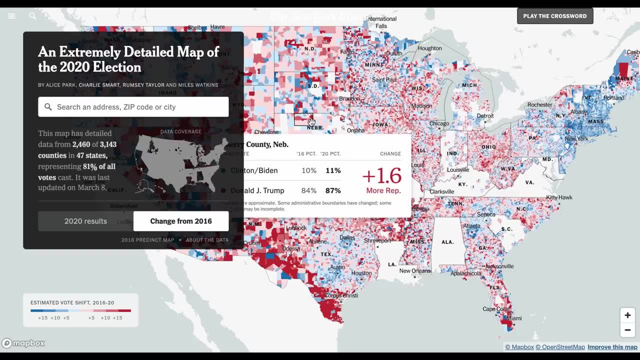 democratic between the two elections. this means that, on this change from 2016, map places that appear red, for example, may not have actually had a majority of voters. vote republican just more than in the last election. if you want an idea of how certain parts of the 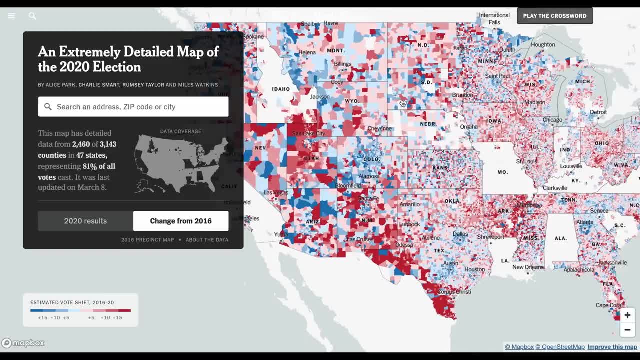 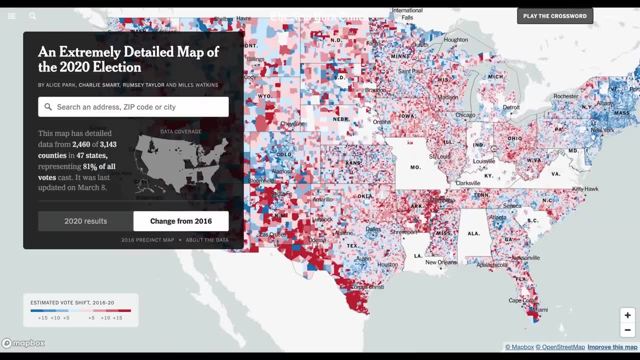 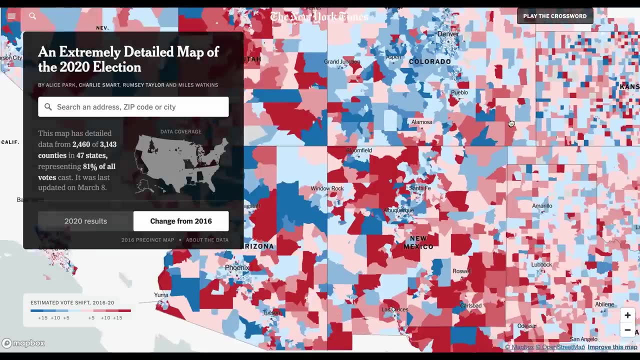 country are trending politically, this can be a useful tool. often people will just look at which states flipped in an election- and states usually flip every year. but this gets far more specific and shows trends even in states that did not flip. for a look at how this map should appear if there is really no change between elections: 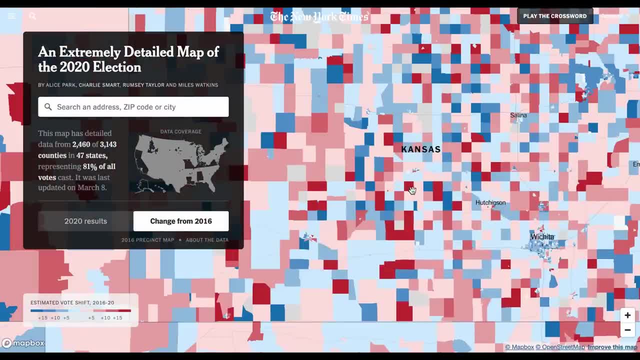 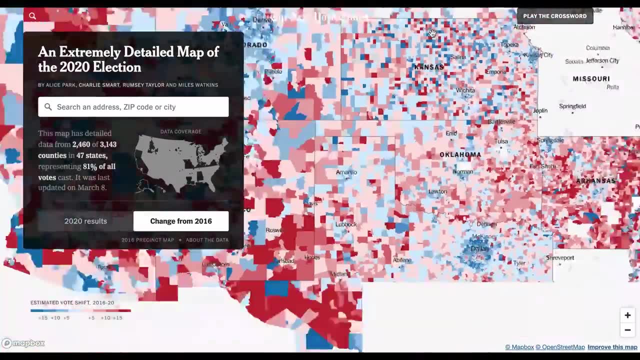 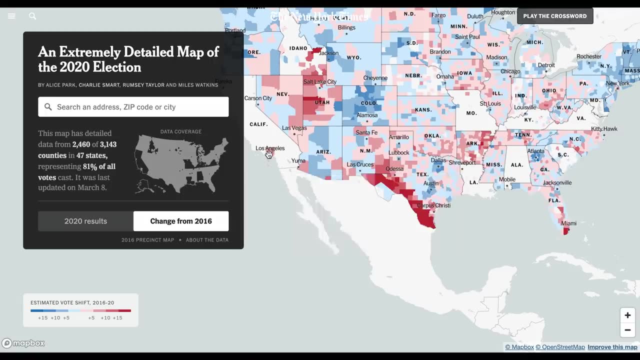 let's take a look at rural kansas. some precincts got redder, some got bluer, but these appear pretty haphazard and random. other areas of the country, though, had clear trends moving in one direction or another. much was made after the election of trump's improvement among latino voters, and indeed through this map you can see. 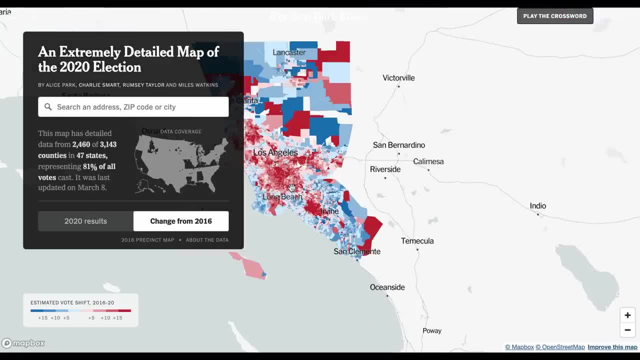 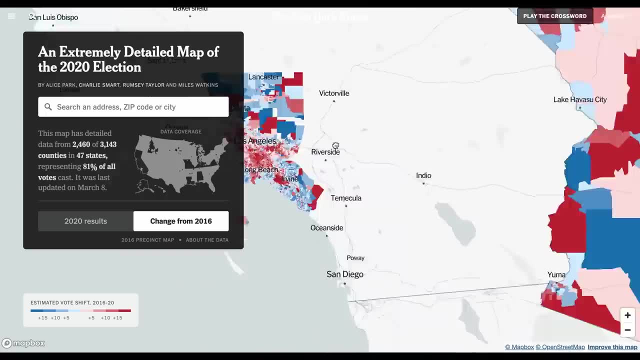 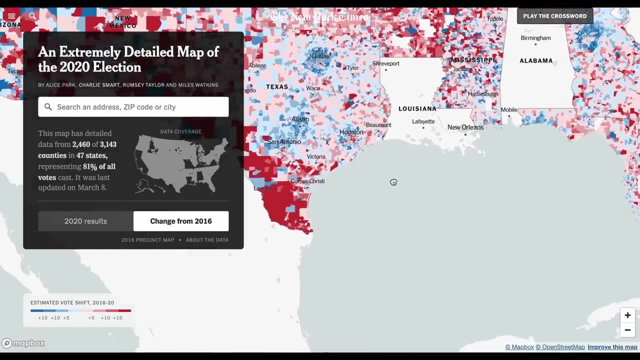 that areas with large latino populations, such as los angeles, grew significantly redder, even though in the case of la, it barely made a dent. other areas home to many latino americans, such as south texas and the miami area, also turned redder, turning two democratic strongholds into pretty. 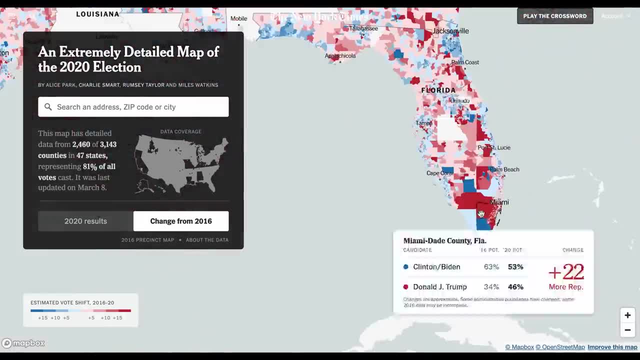 competitive areas. the results in miami are particularly striking for democrats to win such a major urban area. for example, in canada, the surrounding capitol is not the most looked-after population. this is the most likely to be the case. but i want to point out a few things about the. 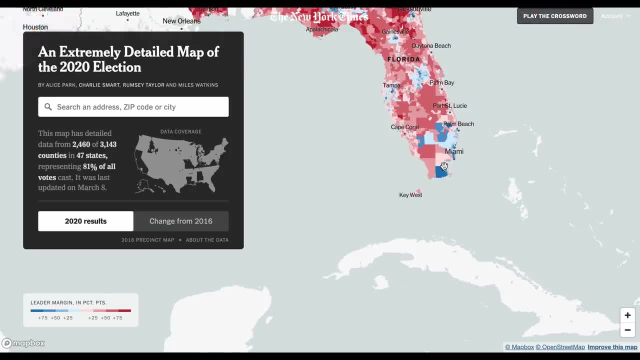 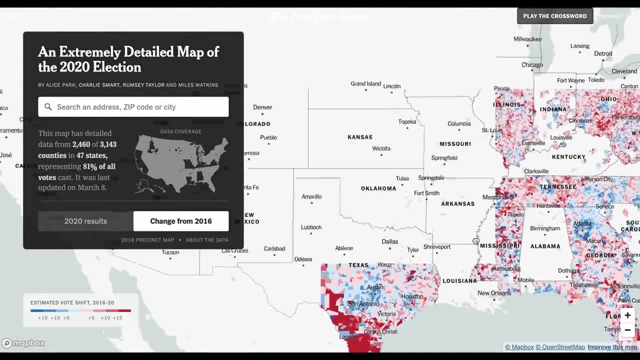 places where the party typically does best, by a relatively slim margin of just 7%, was quite a surprise and likely helped cost Biden the state of Florida. Trump also appears to have further solidified the Republican grip on the states of Utah and Arkansas. 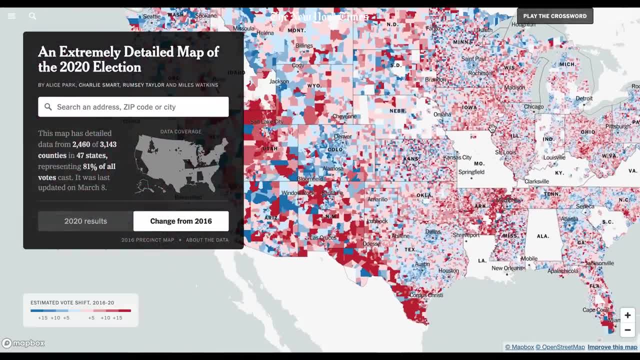 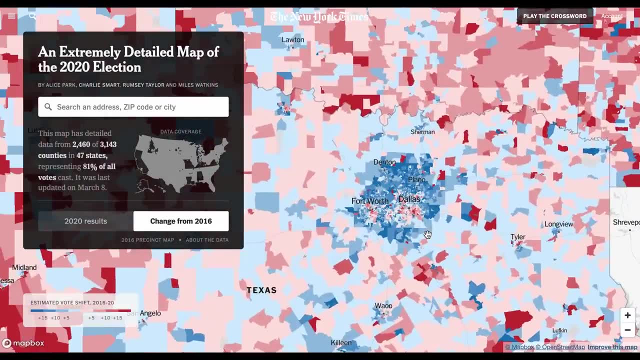 However, other than Miami, Biden did about as well as Democrats typically do in major cities and more than made up for losses elsewhere with decisive wins in the suburbs. If you look at a lot of the cities on this map, you can see what looks sort of like a donut surrounding them. 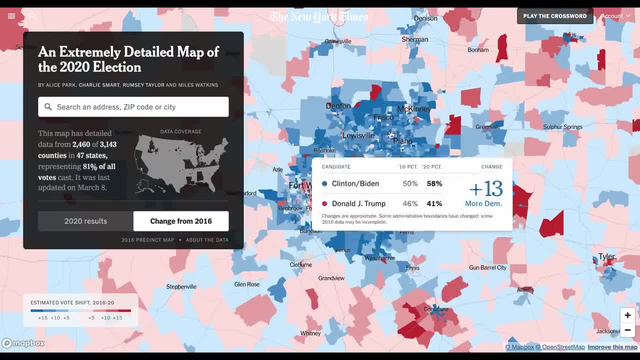 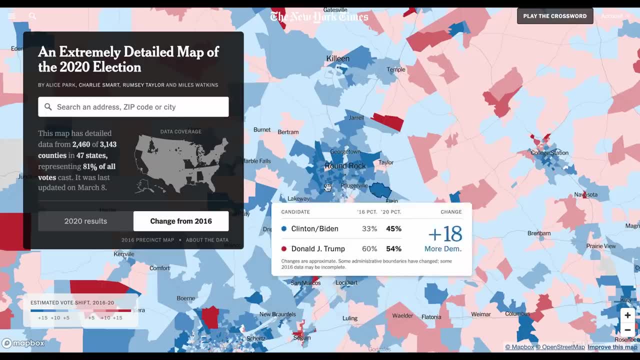 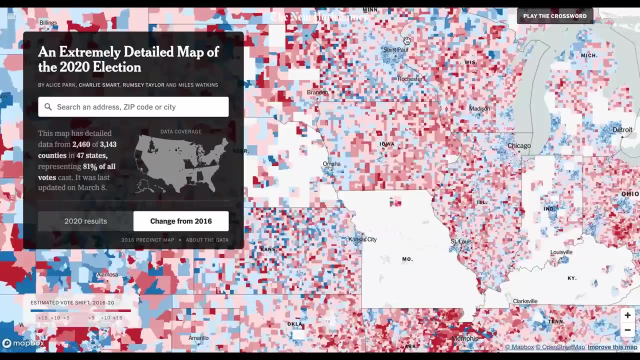 This is a result of the cities themselves getting either slightly bluer, redder or staying about the same compared to 2016,. while the suburbs got significantly bluer, creating a wide blue ring around many of them, This blue suburban donut appears around nearly every city on this map. 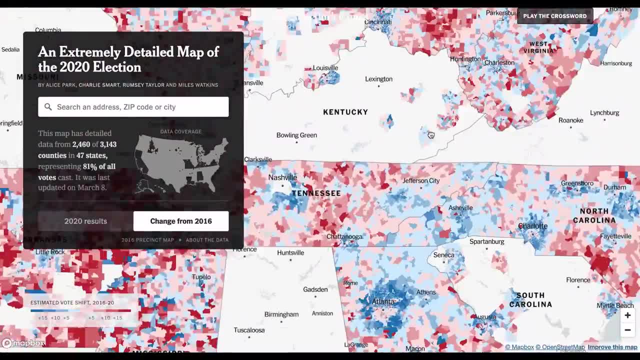 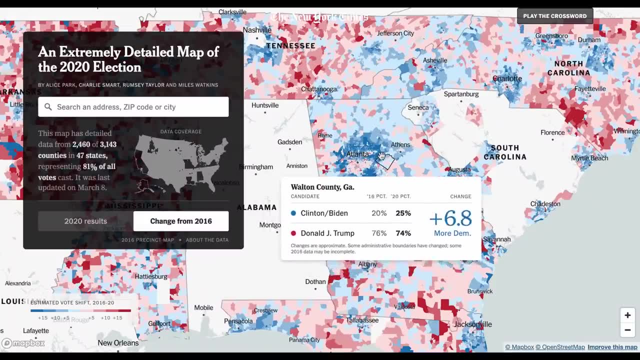 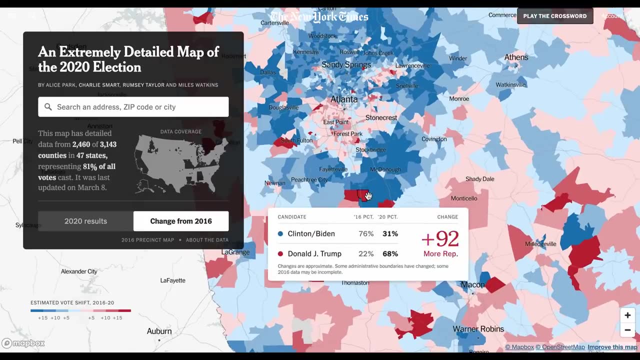 and is even more consequential because suburbs are typically very politically competitive. If you look at a state like Georgia, which saw Biden win a narrow surprise victory, this is extremely evident in metro Atlanta, While he may not have picked up every suburban, county candidates need to win states, not counties. 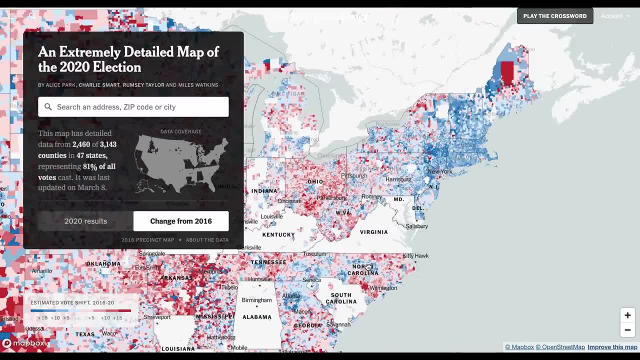 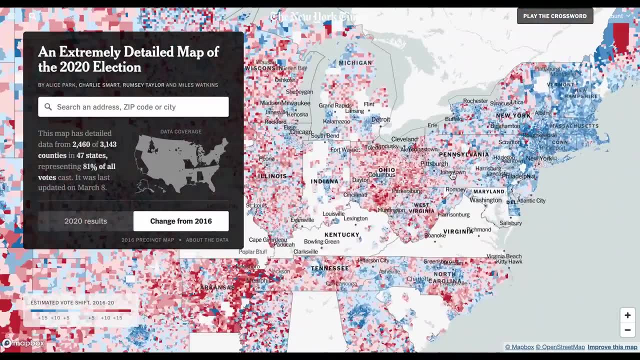 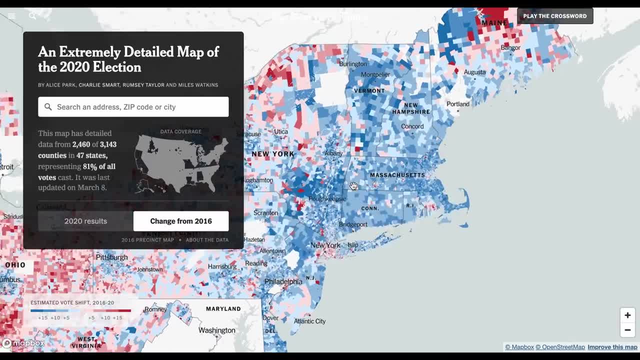 he outperformed Hillary Clinton's margins in the suburbs. he outperformed Hillary Clinton's margins in the suburbs. he outperformed Hillary Clinton's margins in the suburbs. The region is already a Democratic stronghold, so it won't do much but make the state safer for. 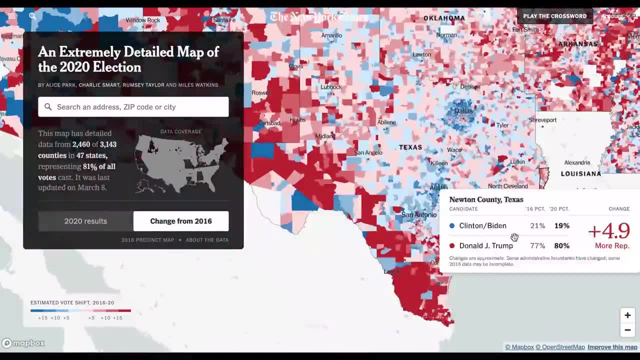 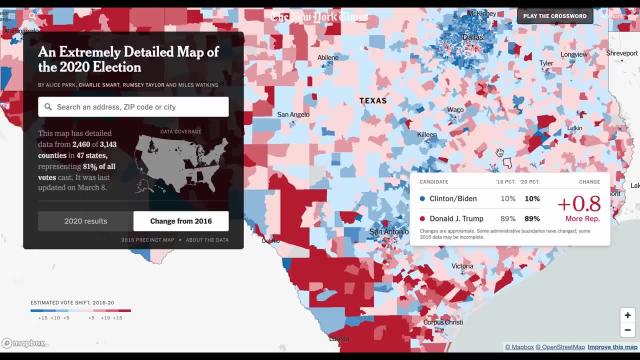 Democrats, but it's interesting nonetheless. Finally, there's been lots of talk of Texas flipping for the Democrats sometime in the future, and while Republicans did better in 2020 in South Texas, other parts of the state located around the edges of many of its major cities did get. 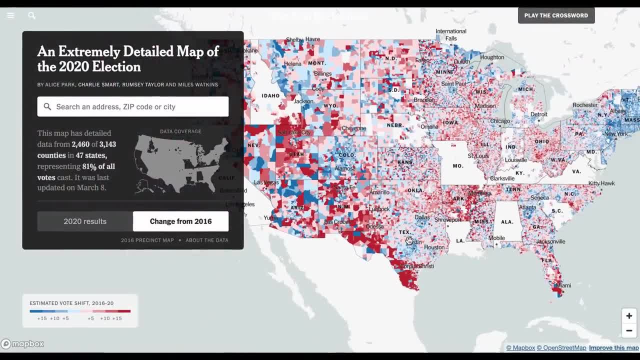 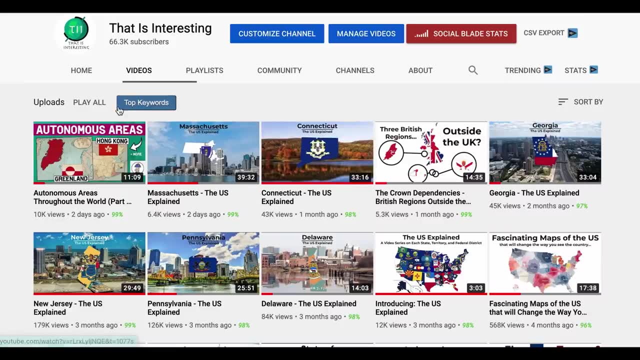 bluer, which, in my opinion, will make it an interesting state to watch. If you're interested in US geography- which, if you watched this far, it would seem that you are- I have a series called The US Explained, where I make an in-depth video on the geography, history and culture of each. 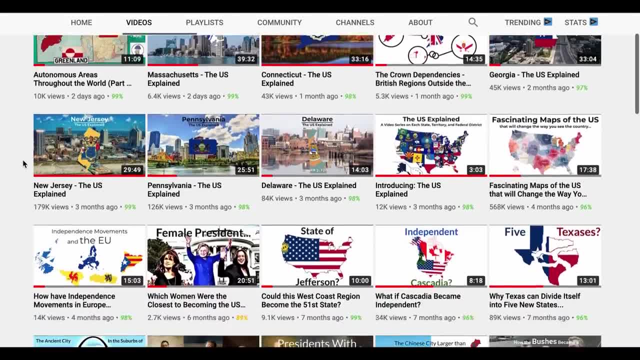 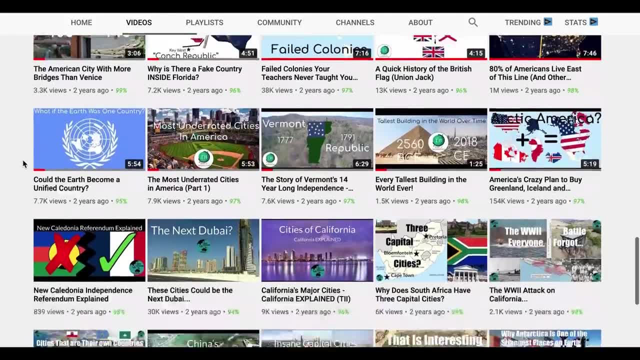 state, territory and federal district in the United States. If you're more interested in international geography, I have plenty of videos on those topics as well. Also, please check out the TII store, where you can purchase some great, That Is, Interesting merchandise and consider. 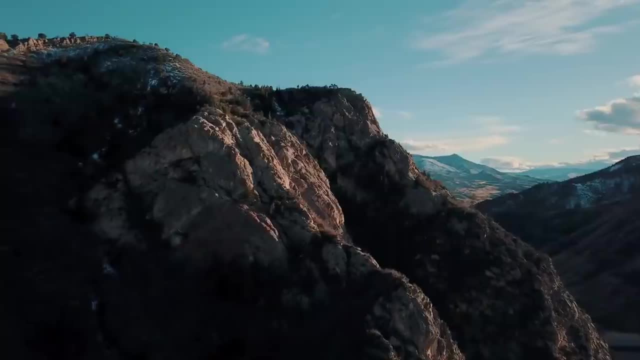 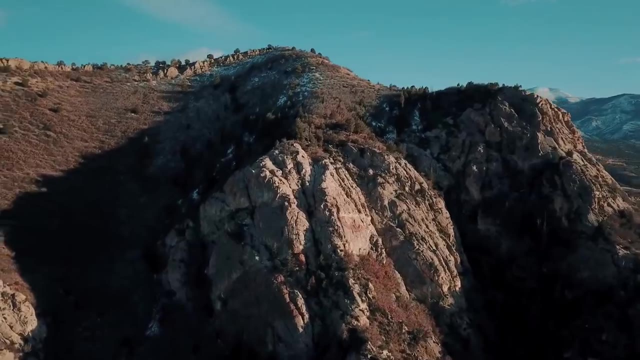 joining my Patreon. Both are great ways to support the channel. My Discord server is a great place to connect with other viewers and talk about topics that you're interested in. Links to all three will be in the description. Thank you for watching this video.